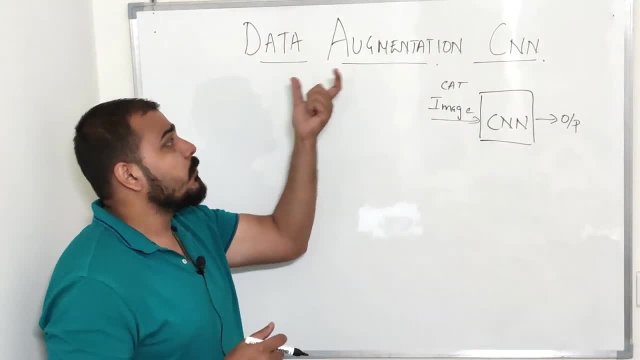 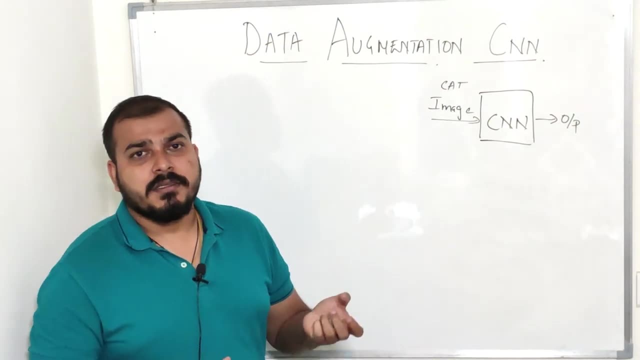 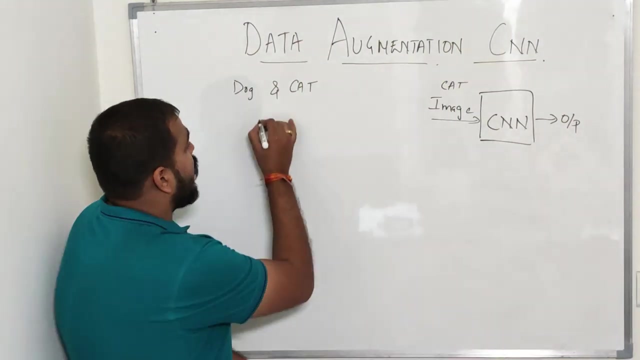 So let us go ahead and try to understand what exactly is data augmentation? Now, guys, you know that whenever we are solving CNN right, we'll basically be having data set of images. Suppose I have dogs and cat images, So over here- usually dogs and cat images. 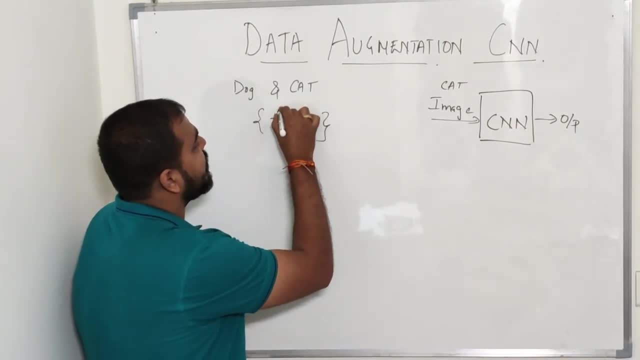 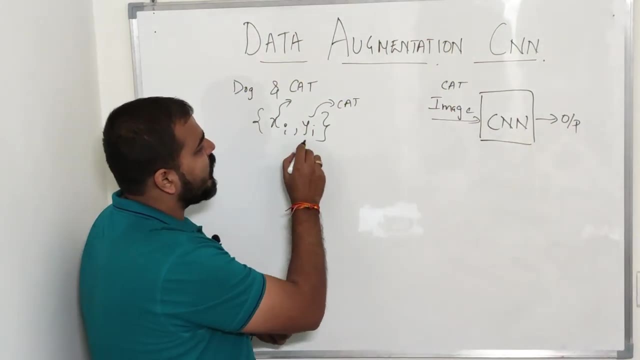 I can also write it as X of I, Y or Y Over here. I can say that if the X image is cat, my output- Y or Y- will be cat. Or if the X image is basically dog, can basically say that my output is dog. now understand what exactly data. 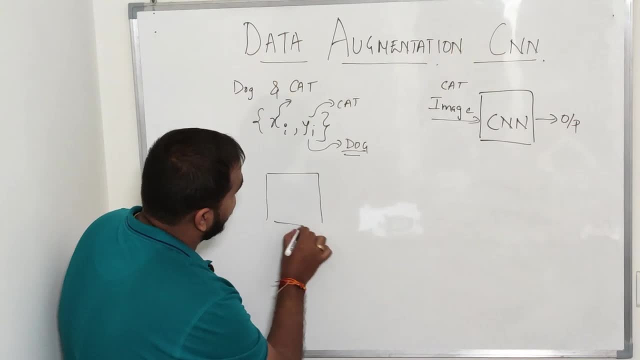 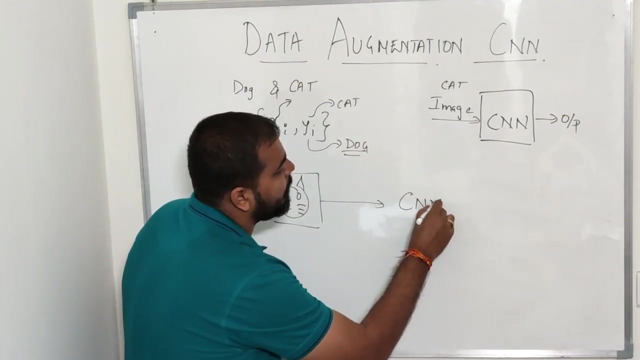 augmentation. basically say, now suppose this is my cat image and I'm extremely sorry about the image, just try to understand what I'm actually trying to draw. so suppose this is my image, okay, and this particular image is basically going to a CNN, right, a CNN that is convolution, neural network. and finally I 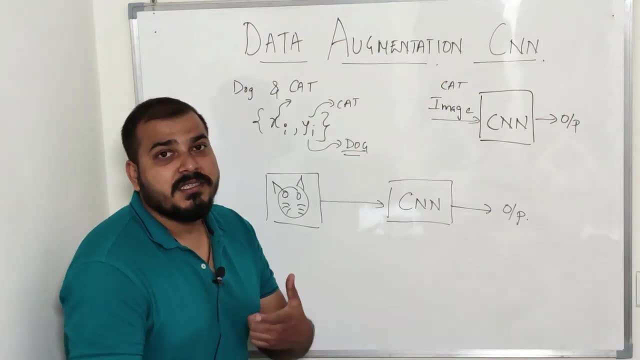 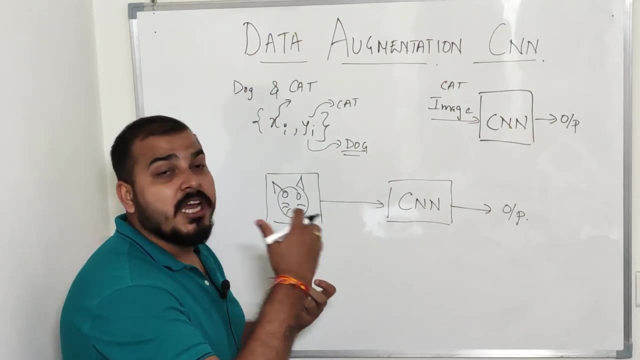 get the output saying that the image is a cat or a dog. now, what does data augmentation helps us to do? data augmentation: with the help of data augmentation, I can transform this particular image into different, different kind of images. okay, now, when I say different kind of images, the output. 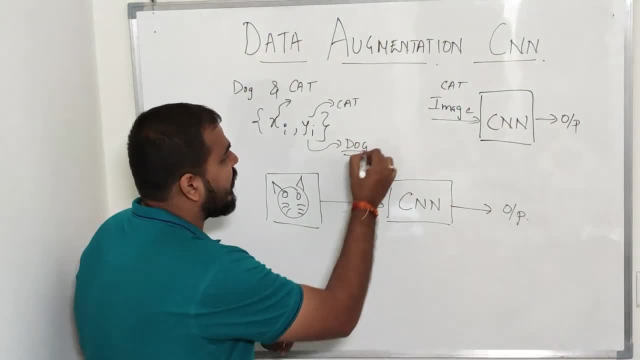 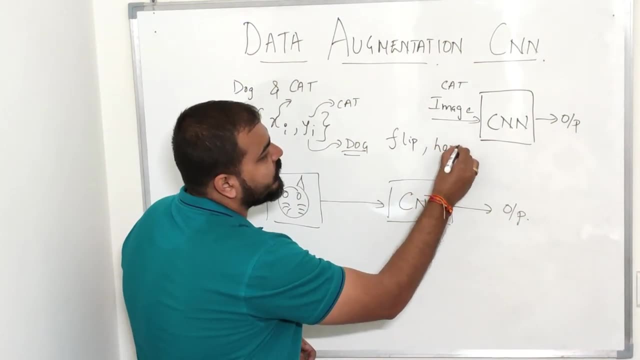 will be cat only, but some of the transformation. what are the transformation that I can do? that is called as flipping. I can flip this images. I can also do horizontal shifting. okay, what does horizontal shifting mean? or I can also perform vertical shifting. okay, I'll just discuss about this. what is horizontal shifting and vertical? 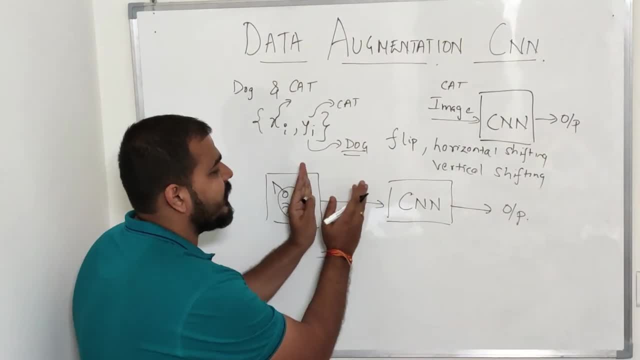 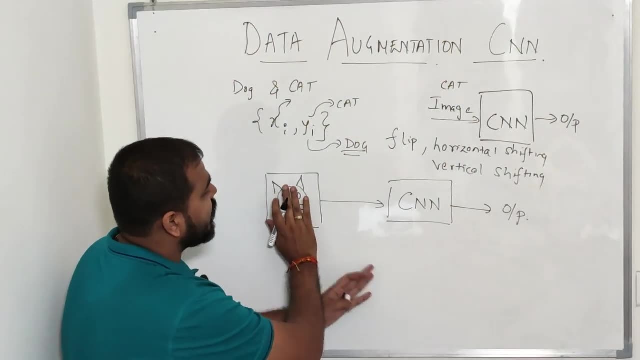 shifting. suppose this is my cat image. I can just move this image little bit at the right or little bit to the left. okay, there is also called as flipping. I can invert that particular images like horizontal flipping. I can invert it like this: okay, or I can also do vertical flipping, vertical flipping, what it will. 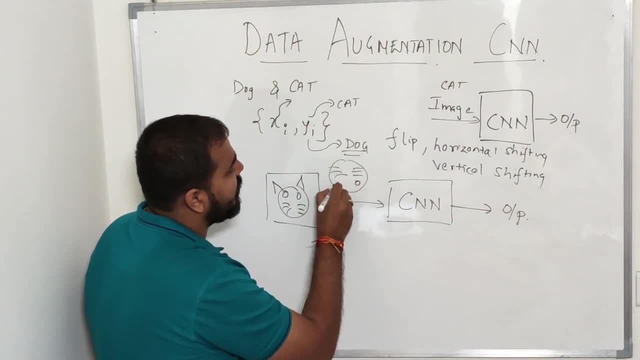 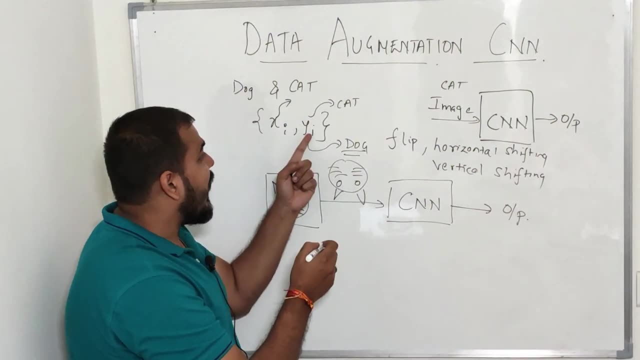 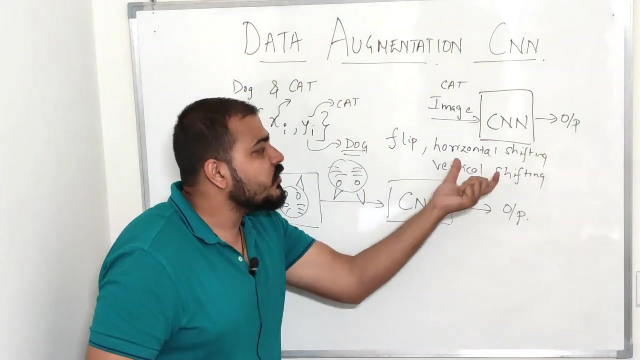 do is that it will just inverse that particular image. now, my eyes will be here, my ears will be here, right, always remember when I'm making this combination, the Y of I, the output will be same, but I am transforming this image is into different, different stylings. you know, by applying flipping, horizontal shifting, 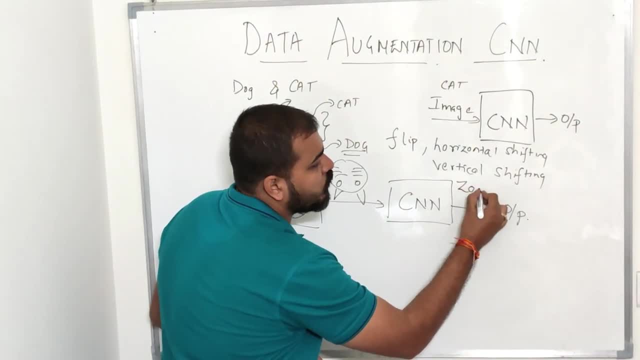 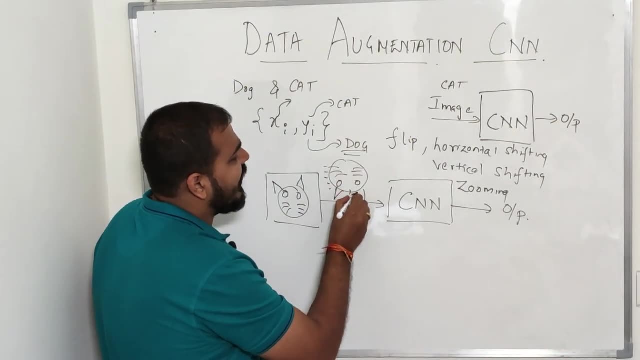 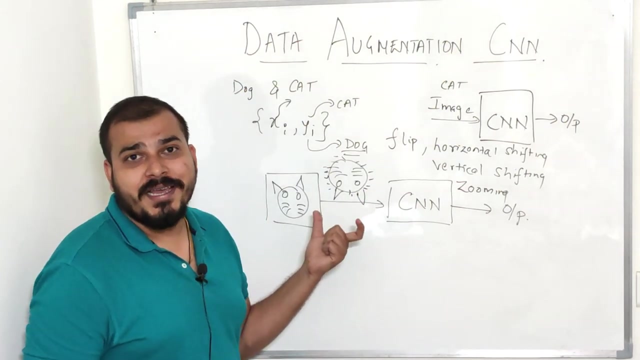 vertical shifting. you know I can also zoom it. I can also zoom the image, zooming like I can do a 20 percent of zoom. I can also add some noise. you know I can add some more noise into this particular images, some, some points, right. so different kind of things we can actually do with the image wherein we are just transforming the image: the same image. we're just trying to describe the image. Where can we transform the image? You see now, you see some of the- yeah, the objects. we can actually mount the image, the same image that we have launched. that is exactly the same we can. 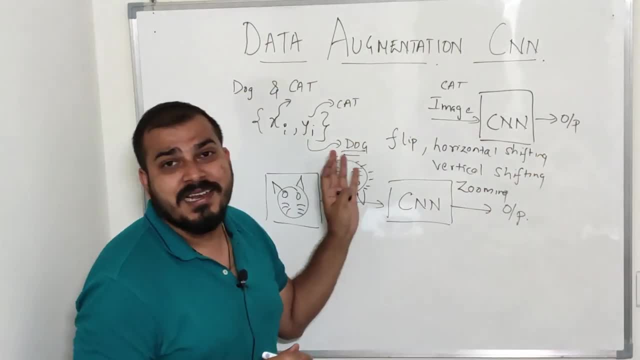 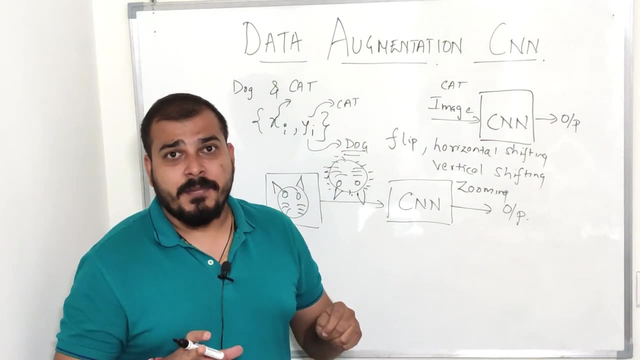 transform it. so different types of steel images. you know, I can change the image, the that we have here transforming, by using this particular properties like flipping, horizontal shifting, vertical shifting, zooming, zoom out, you know, and different, different categories are there. Now I'll also be showing you how this. 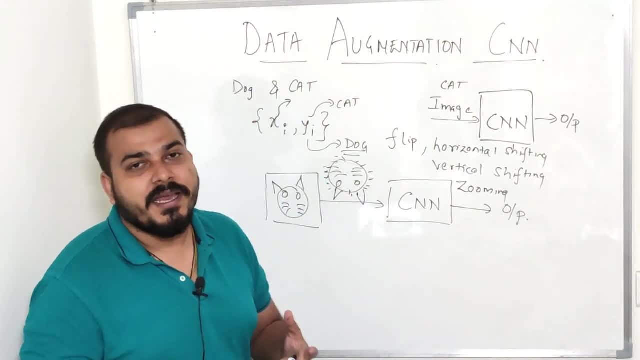 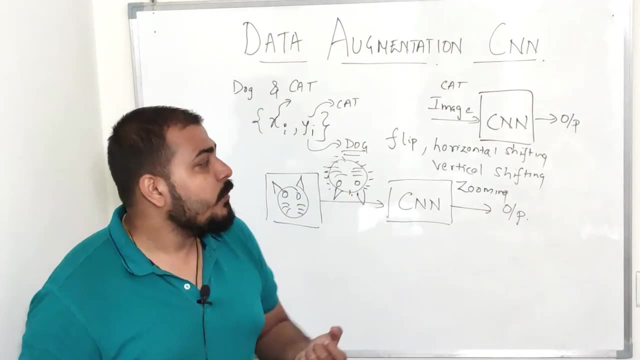 can be implemented when I'll be doing the CNN implementation. over there There is a very good library regarding data augmentation and I'll show all these particular examples with the help of Keras, So at that time you will be understanding how the same image can be transformed into multiple images with 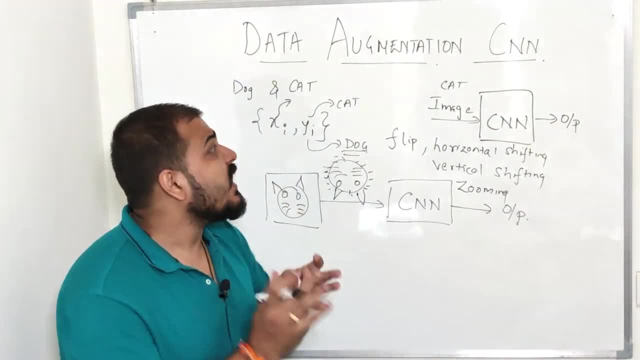 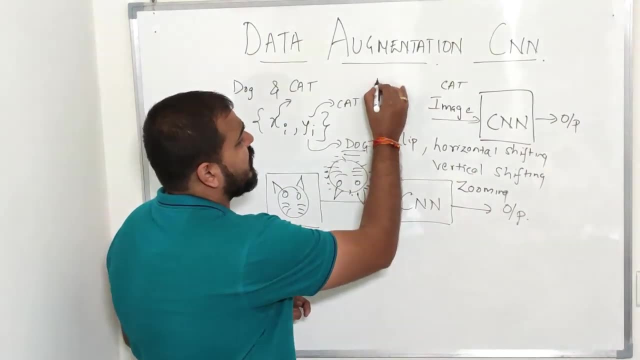 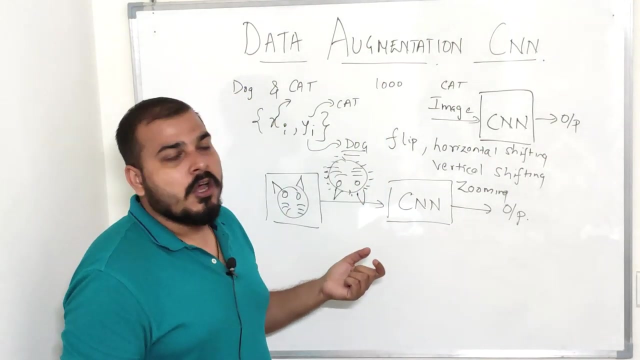 the same output. Now in to understand why exactly is data augmentation very, very important? Now remember, guys, suppose if you have very less number of data sets, I have just, you know, thousand images, right? I need more images to, suppose, categorize some animals, right? so suppose I have thousand images of cats. 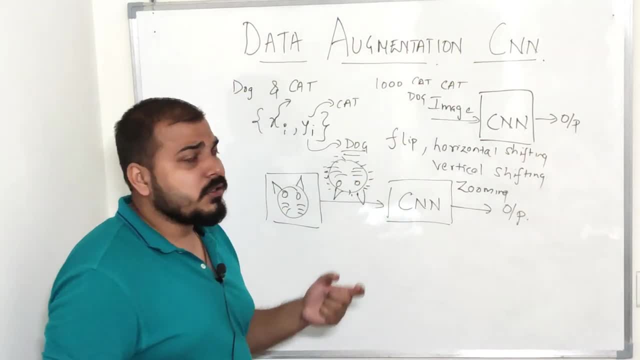 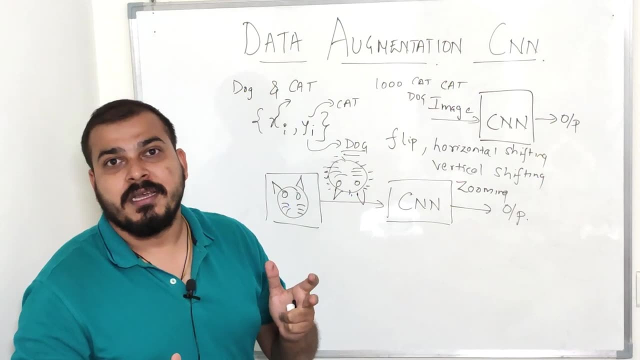 and dogs, right, and I suppose if I take this- cat images, if I do this data augmentation, I'll be able to get many more images, all different, different kind of images. We basically tell a term which is called as invariance. we'll be able to add some invariance into. 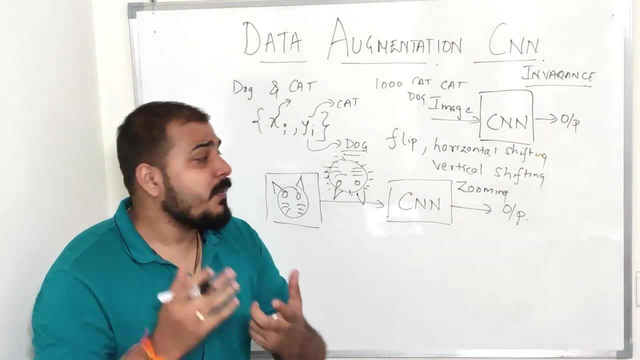 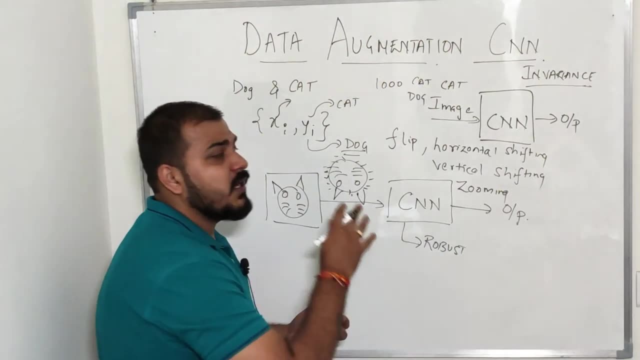 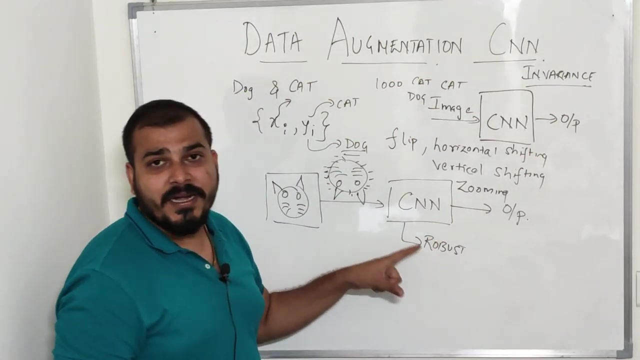 the images, some different styles, and always remember, guys, whatever CNN model we are actually creating, it should be very, very robust. that basically means, if the, if the cat looks like this, if it is flipped vertically, then also our CNN should be able to predict that: yes, this is a cat image. Now, this data. 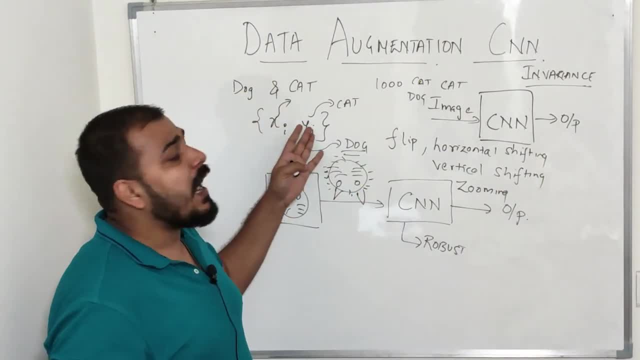 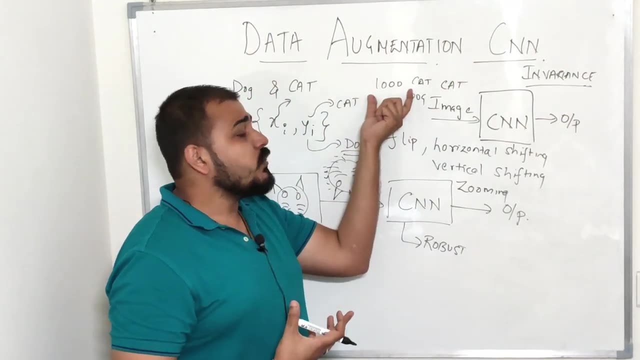 augmentation helps us to create many more images with the same output and because of this you'll be able to get various data set. the data set increases, suppose, if you have thousand images right and if you try to do data augmentation with ten different parameters, many number of. 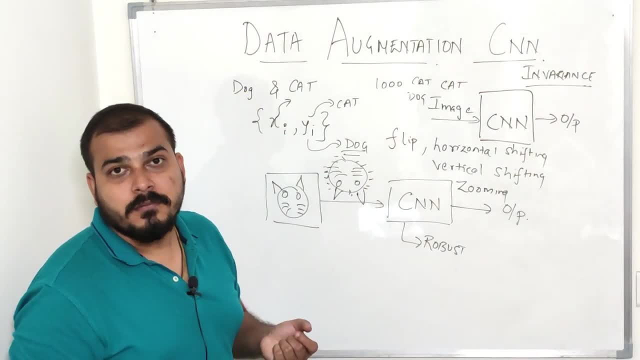 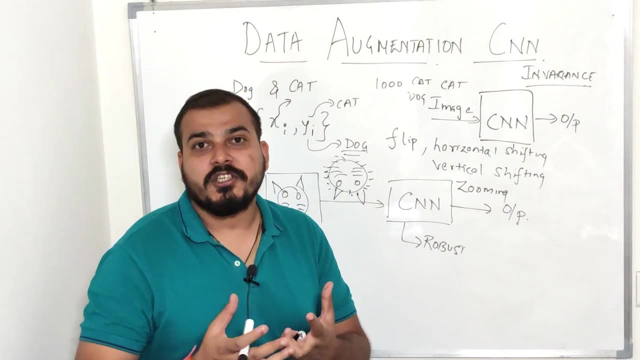 images will be getting created of the same cat. you know, suppose one cat is there, if I apply this, it is actually creating ten more images. in short, so this will actually help you to get more data set and, by default, your CNN will become more robust because, in the same way, CNN will be able to create more data sets and, by default, your CNN will become more robust because, in the 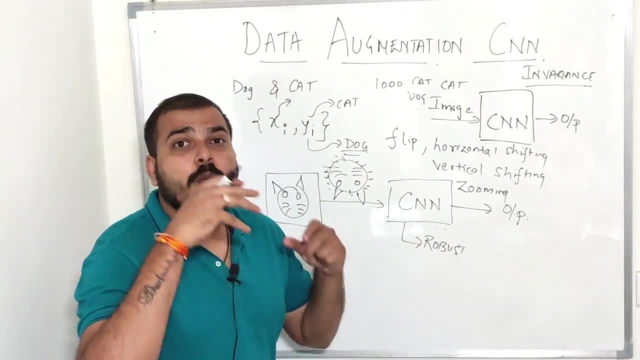 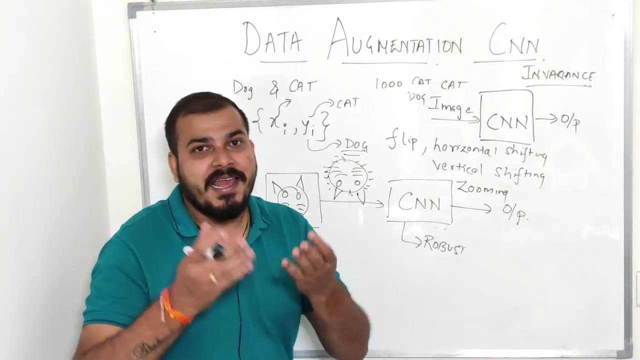 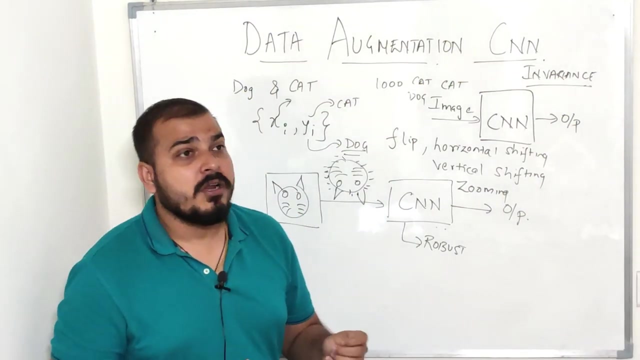 CNN. we have filters in the convolution layer. those filters will be able to do edge detection. vertical edge detection will be trying to take more and more features from this images and hence it becomes robust and it will be able to give a very good prediction. so this is what data augmentation is all about it. 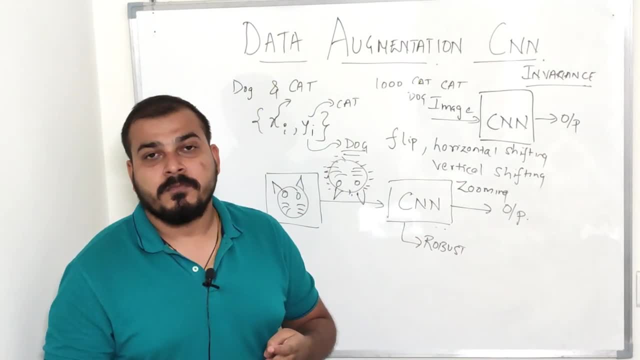 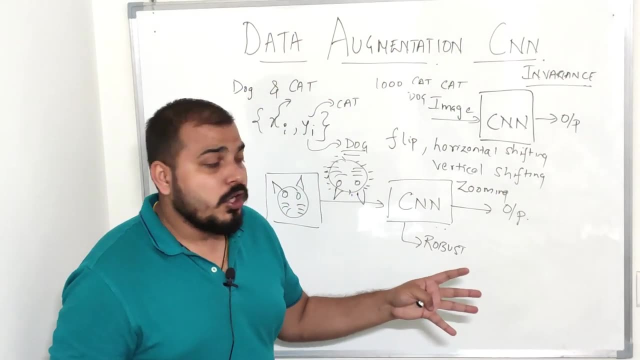 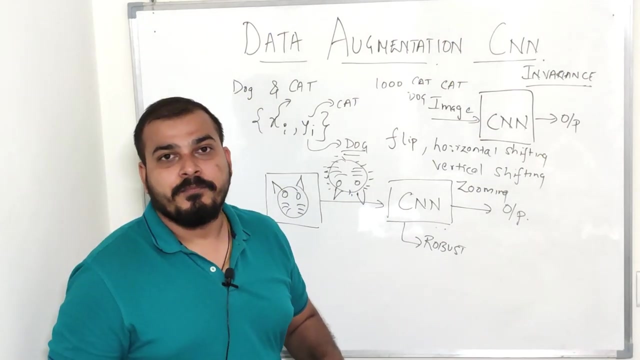 is actually capturing invariance by creating more images. you know, internally it will not create and save it somewhere, but when we are actually applying into data augmentation, you know we, we, when I'm giving this one image, is similarly, by applying this transformation, we will be giving ten images to the CNN. so suppose, if I'm doing, 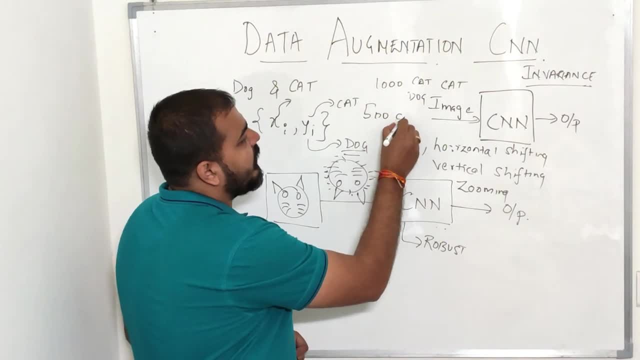 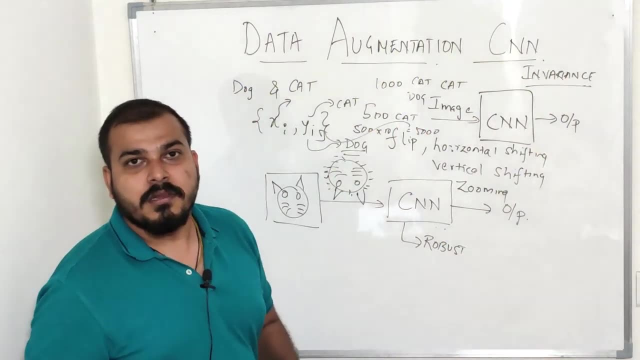 ten different type of transformation. if I have 500 images of cat, this will in turn become 500 into 10, that is, 5,000 images with the same output: cat. now, because of this, the CNN will be robust and it will be able to easily determine. 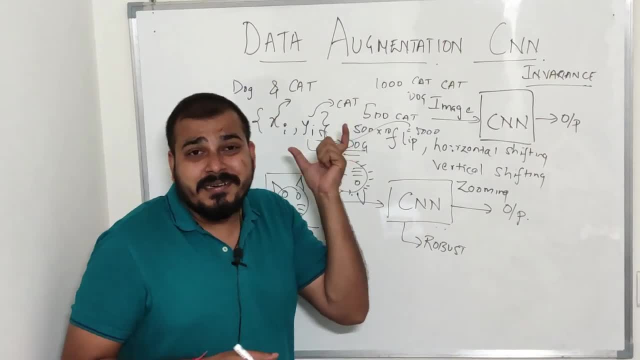 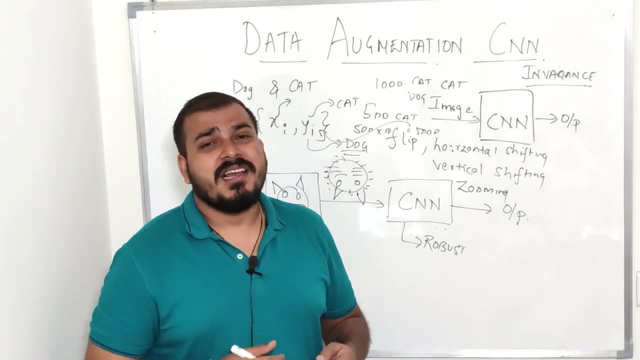 this right. so this is a very important step and this is the last step of data augmentation. in CNN there is also after the max pooling layer. there is also called as a dense layer, which is just like a fully connected layer, and you know, once the fully connected layer is connected. 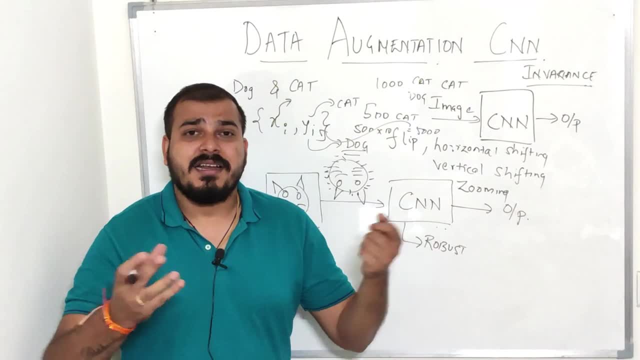 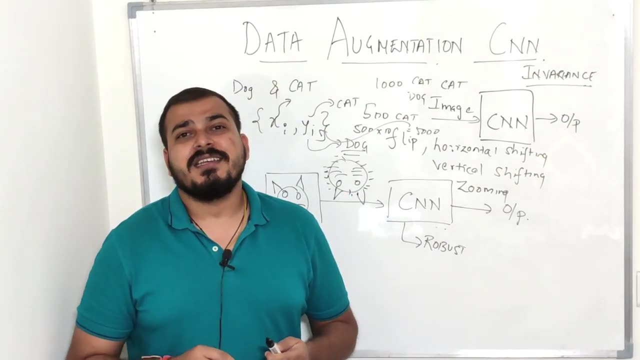 in the back propagation, all the weights, all the filters will get updated and that is how a CNN is basically created. in my next video, I'll be showing you a very good practical example how you can easily create a CNN neural network with by taking a very simple example. usually you will require GPU to run, you know. 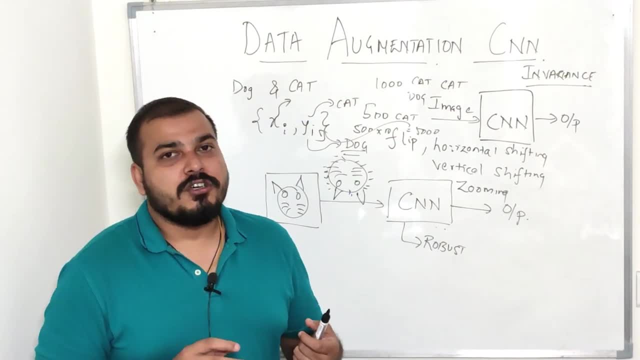 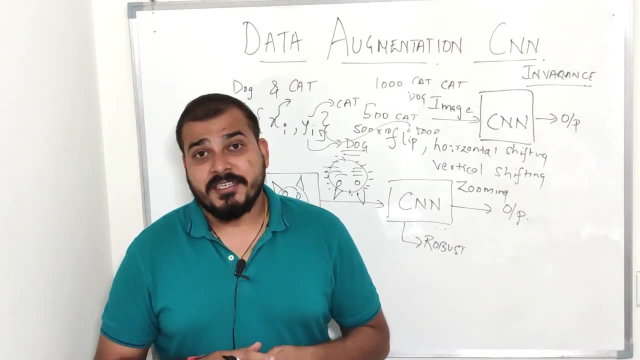 CNN convolution neural network when you have many more images. but I'll try to show you, with the help of my local system, only where you will be able to run that particular code in 30 minutes. so I'll I'll show you that in my next session. so this is all about the video regarding this, and this is tutorial 25th.